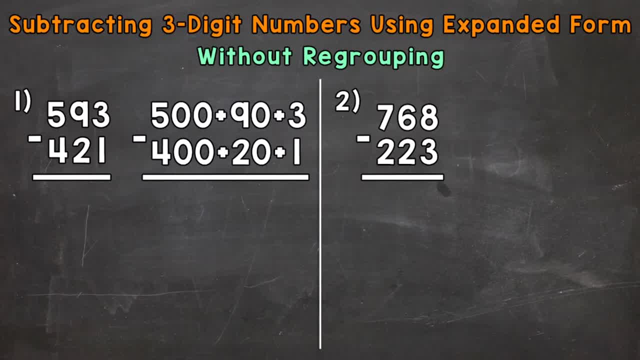 into expanded form. but let's review here. So 593 equals 593.. Well, we have a 5 in the hundreds place, so that represents five hundreds and has a value of 500.. We have a 9 in the tens That represents nine tens and has a value of 90.. 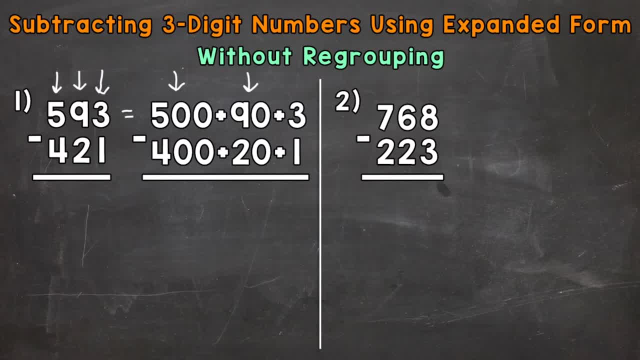 The 3 is in the ones place. It represents three ones and has a value of 3.. As far as 421, well, 421 equals. the 4 is in the hundreds place, so it has a value of 400.. The 2 is in the tens place, so it has a value of 20.. 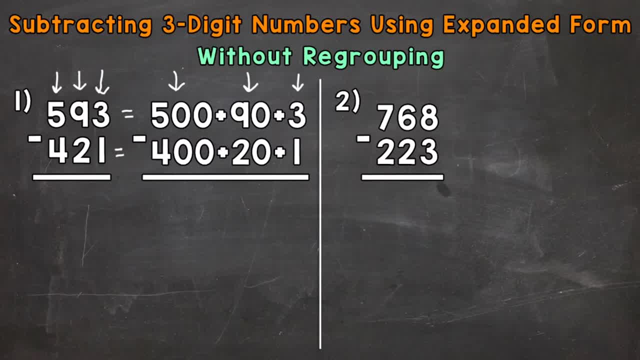 And then the 1 is in the ones place and has a value of 1.. Now that we have those in expanded form, we can subtract. Now when we subtract whole numbers we always start with the ones place. So we have. 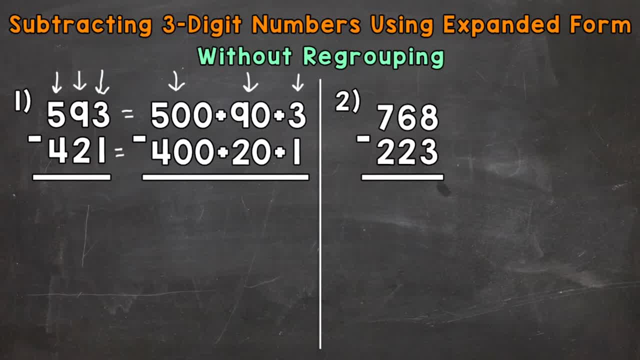 3 ones minus 1 one. That gives us a 2. in the ones We bring our addition sign straight down. Now you may be wondering why we have addition signs throughout a subtraction problem. Well, those addition signs are part of the expanded form. 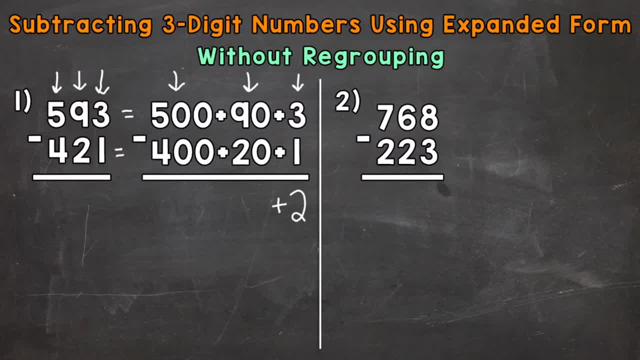 We are still subtracting as we go throughout the problem, so don't let the addition signs fool you. At first our answer is going to be in expanded form, And then we'll change it to standard form. So let's continue subtracting and move to the tens place. 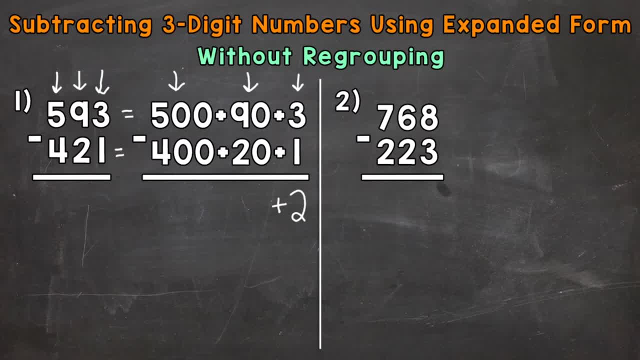 So we have 90 minus 20.. That's going to give us 70.. Bring our next addition, sign down and then subtract the hundreds, So we have 500 minus 400.. That's going to give us 100.. And that's our answer in expanded form. 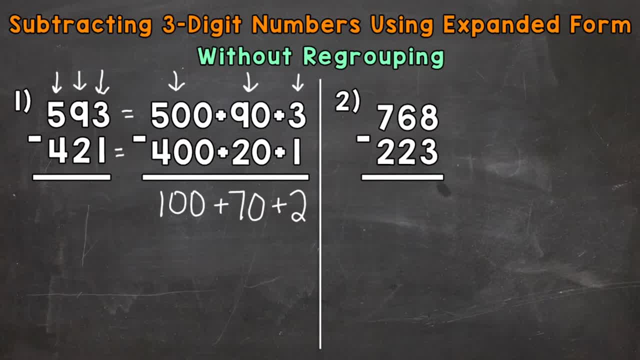 So we have 100 plus 70 plus 2.. So let's change that to standard form. So just writing the number, like we usually write numbers. So we should have a 1 in the hundreds place, a 7 in the tens and then a 2 in the ones. 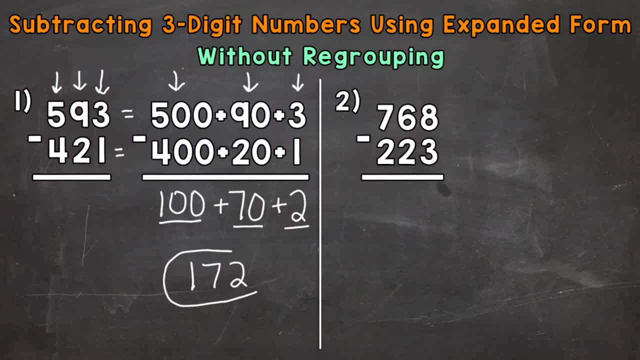 So 172.. And that's our final answer. Let's solve this to the left as well to see if we get the same answer. Start with the ones We have: 3 ones minus 1, one That was represented right here. 3 minus 1 gives us 2.. 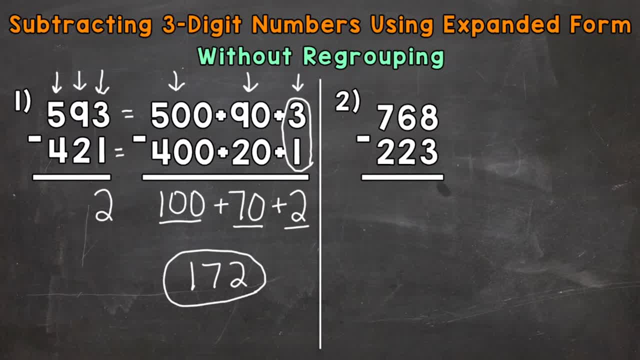 Let's move to the tens, where we have 9 tens minus 2 tens- That was represented right here. So 9 minus 2 gives us a 7 in the tens place. And then lastly the hundreds, So 500 minus 400.. 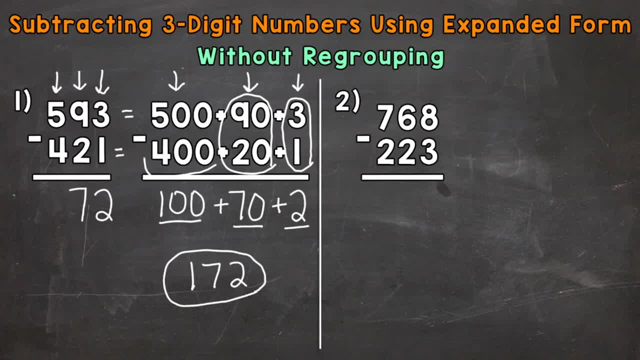 That was represented right here as far as the values of those digits. So 5 minus 4 gives us 1. And we get 172 over there as well. Let's try another one and move on to number 2.. So we have 768 minus 223.. 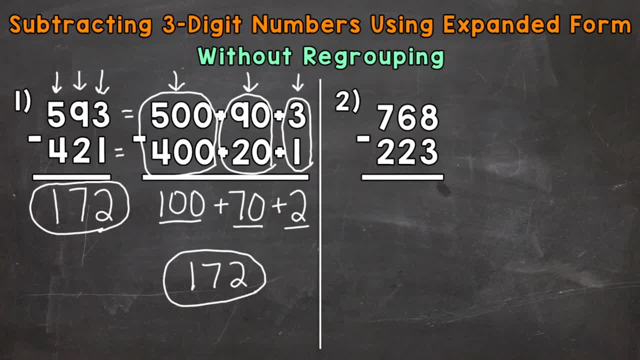 First thing that we need to do put these numbers into expanded form, So show the value of each digit. We'll start with the 7,, which is in the hundreds place and has a value of 700.. Plus, the 6 is in the tens, so it has a value of 60. 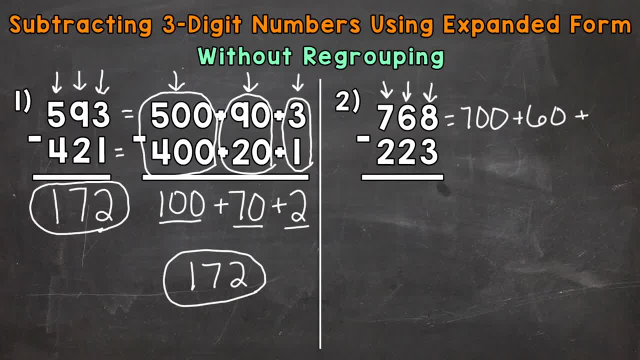 Plus the 8 in the ones has a value of 8.. Minus let's do 223.. So the 2 in the hundreds has a value of 200.. The 2 in the tens has a value of 20.. And then the 3 in the ones has a value of 3.. 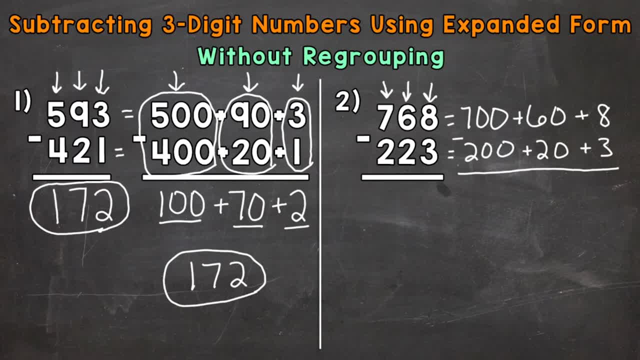 So once we have both numbers in expanded form, we can subtract, Start with the ones, So 8 minus 3 gives us a 5 in the ones, Bring our addition sign down and then move to the tens, So 60 minus 20..